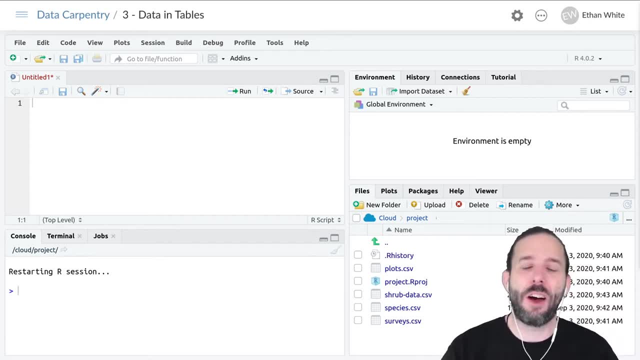 This video is an introduction to the idea of packages in R. Packages are the main way that we share reusable code in R and they're typically a combination of certainly code, but also data sometimes and documentation to tell us how to use the code or how to engage with the data. R has a rich ecosystem of packages for 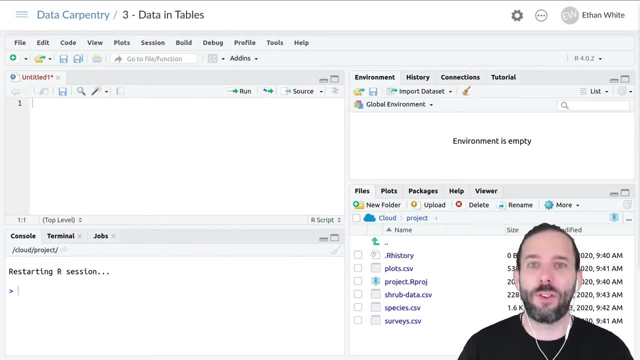 data manipulation and analysis, which is one of the reasons it's popular in biology and one of the reasons we're using it in this course. To download and install a new package, we use a command called installpackages. Now we only need to install a package once. We don't need to install it over and over. 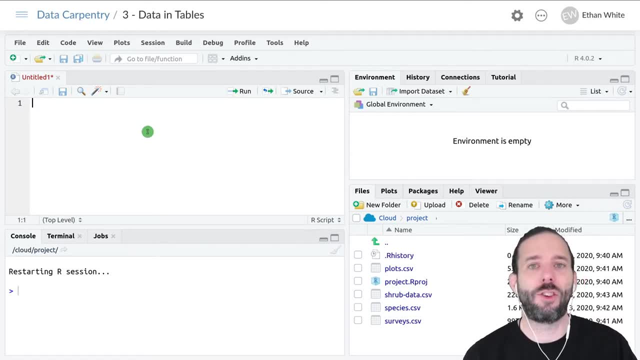 again, and so, instead of installing packages up here in the text editor, I typically install them using the console, and so I'll go down to the console and type the function installpackages. we can see that R Studio is already auto completing it for me, and so I can just click here if I want to. 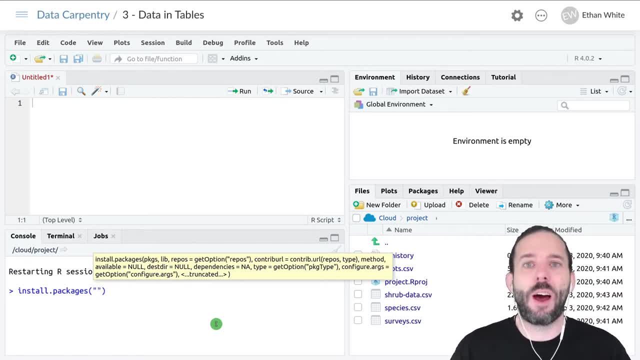 or press tab, and then I need to give it the name of the package that we want to install in quotation marks, and in this case we're going to install the package dplyr, which is distractions. Most of the instructions do. nous-en environ is one of the most popular and powerful packages for doing data manipulation in R. 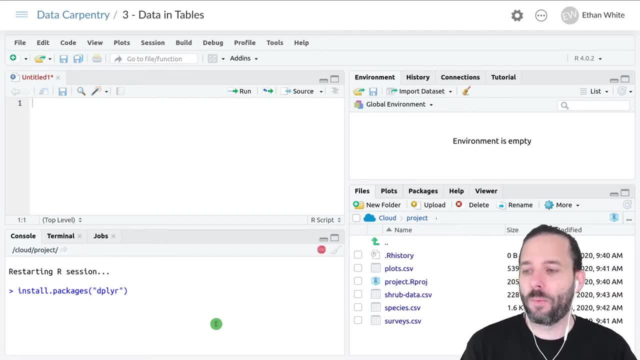 And if so, we. if we do this and then press enter And then wait patiently, We'll see that the package is being installed. now It's telling us where it's being installed to, And then it's downloading not only the package itself but all of the other packages that 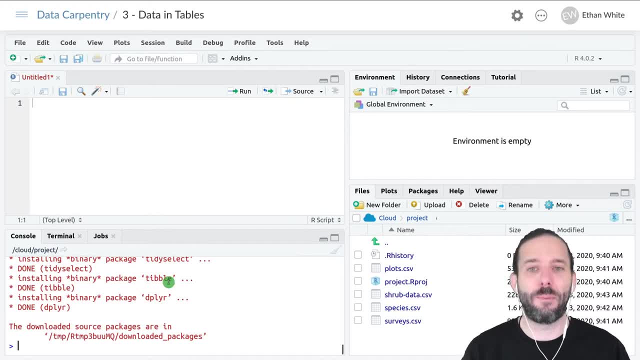 this package depends on and then installing them, And so now dplyr has been installed. Once we've installed a package, it's still not available yet for Using analysis with, And the reason for that is that different packages may have functions that have the 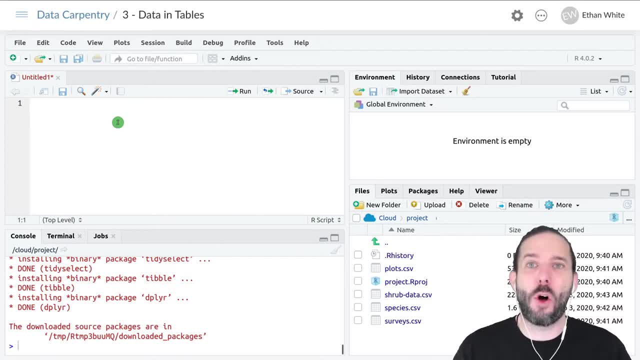 same names, And so we don't want to have to worry about all of the packages we've installed. every time we write a piece of code, And so the way that we tell R that we want to use a particular package and the functions and the data that are in it in some code that we're writing is using the library function. 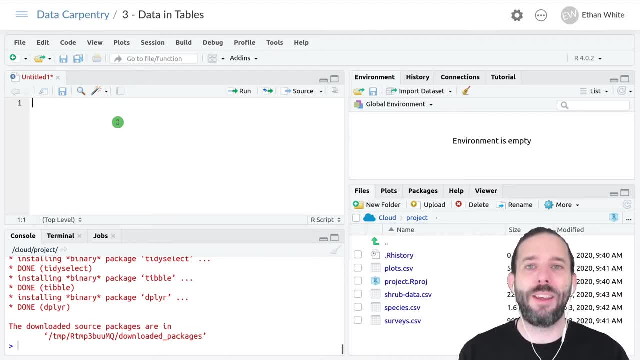 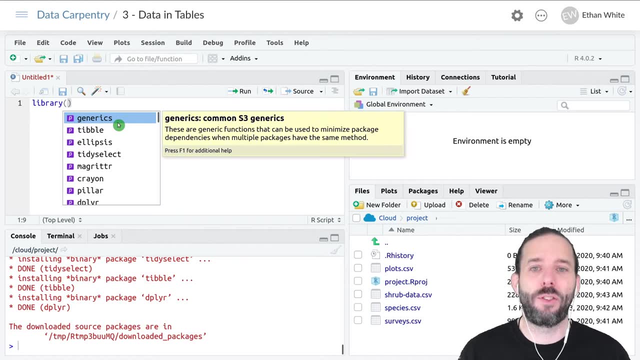 And so at the top of our code, before we write anything else, we type the word the function name, library, followed by parentheses and then the name of the package that we want to load in quotes. And so here again it's dplyr. 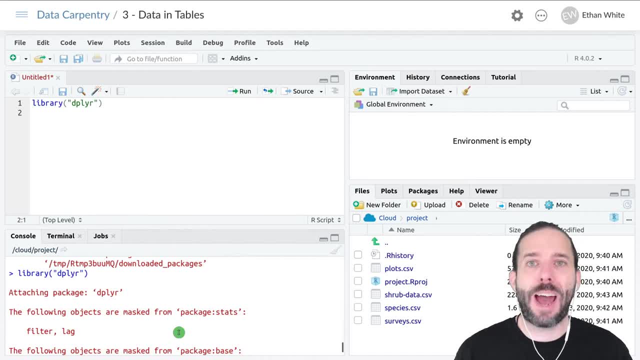 And then we run this code and that will load the package and all of its functions into our, where they can be used. and, as I mentioned a minute ago, sometimes packages have functions that have the same name as other packages and when we load a package we'll actually get some information on that and, in particular, 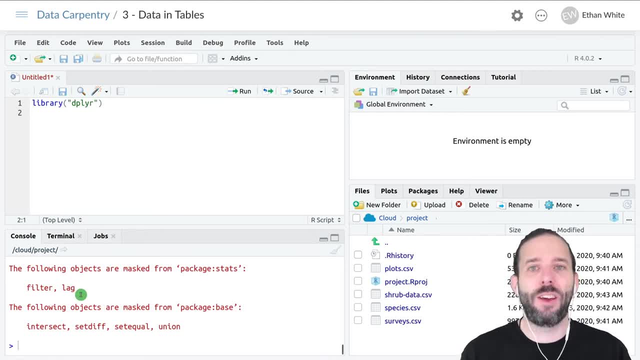 what we see here is that dplyr is masking or it's replacing the functions with the name filter and lag that are loaded by default with its own versions, and also these functions as well, and we'll see examples a little later in the course, where this namespace overwriting becomes important and we really need to. 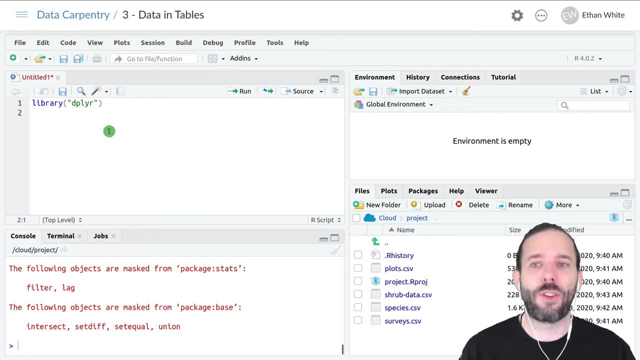 keep track of it, but for now we can just ignore this and start using dplyr, which we'll do in the next lesson. so that's the idea behind packages. we install them once using the install dot packages function, which I typically run down here in the console, but we then load the functions every time we want to.